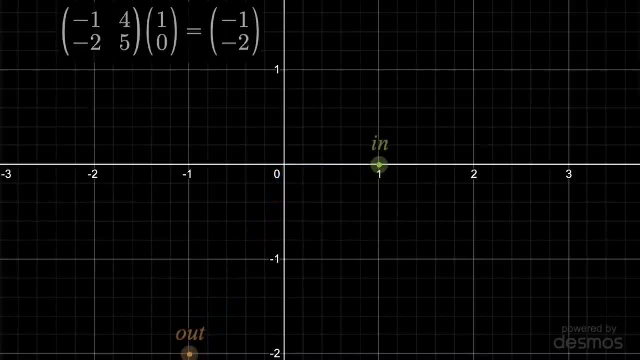 But still, we have an input and output vector and you'll notice that the matrix transformation caused the vector to scale and also rotate. That's usually what happens. Put a random vector in here and the output vector will likely have a different length and angle. 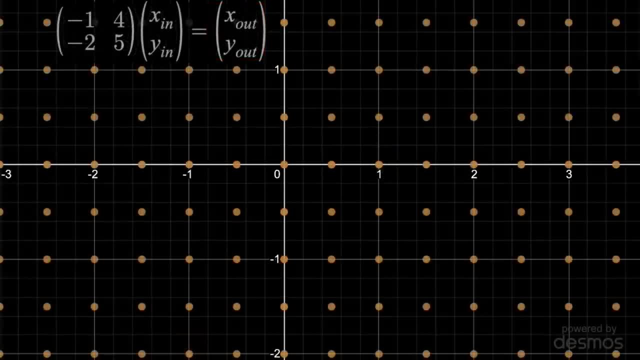 In fact, I'll put a bunch of random input vectors on the screen, or really dots that represent their ends, and I'll apply the same matrix multiplication to all of them at once. These are the new output vectors, and most of them are just scaled and rotated versions. 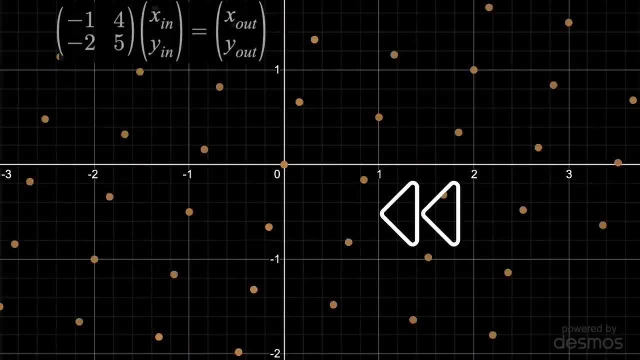 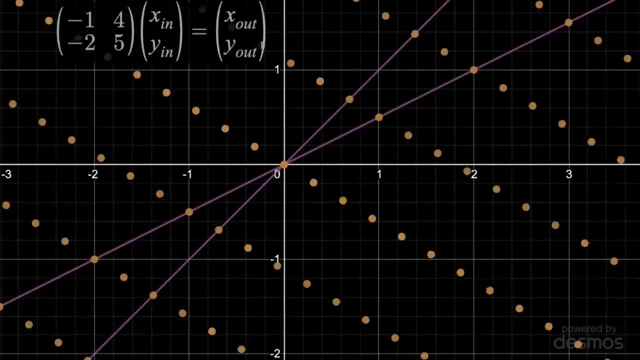 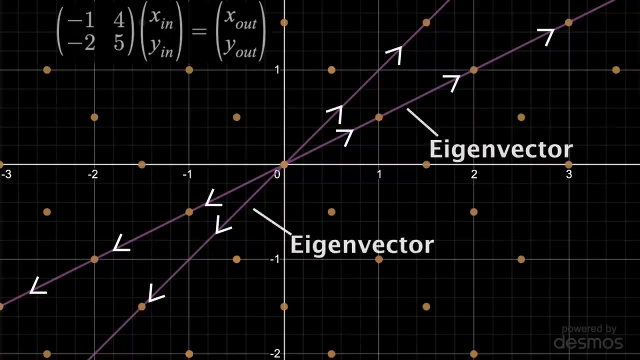 of their associated inputs. But real quick, if we rewind, you'll see that any point on these two lines does not get rotated. Vectors on these lines only get scaled. And when a matrix only scales vectors along some line, that is known as an eigenvector. 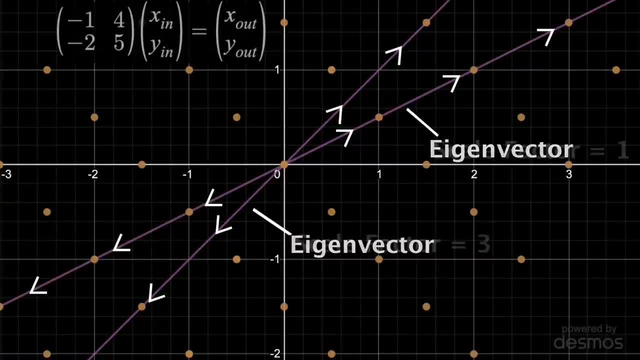 of the matrix. So let's see what happens. Let's see what happens. The scale factor, or how much larger the vector gets, is known as the eigenvalue. You'll notice one of these eigenvalues is 1, because when we applied the transformation, 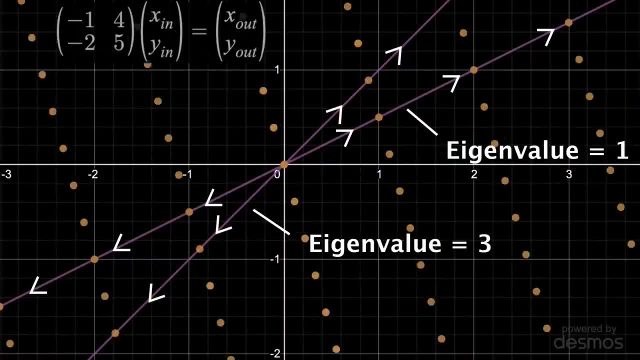 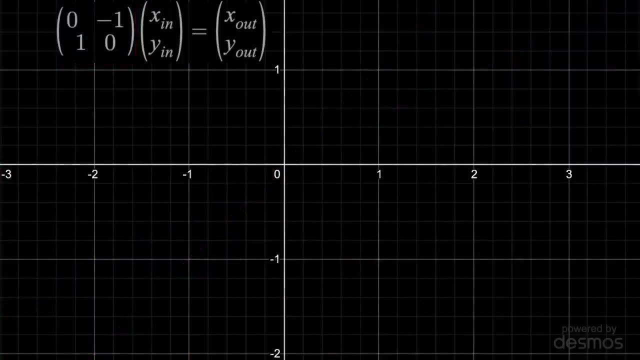 those vectors didn't change in length. If you want to rewind it again, you'll see the dots on the other eigenvector all got 3 times as far from the origin. Now if I change the 2x2 matrix to this, aka a rotation matrix, then any input will be. 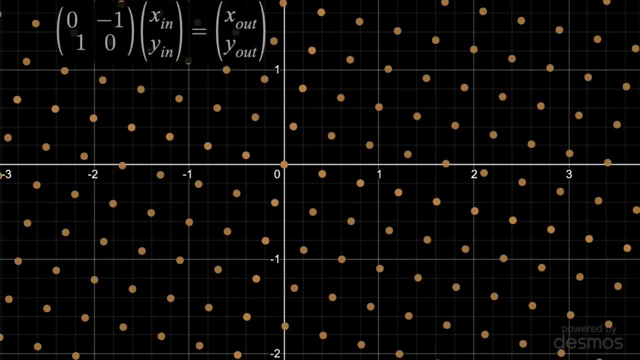 rotated 90 degrees. So if I change the 2x2 matrix to this, aka a rotation matrix, then any input will be rotated 90 degrees. So if I change the 2x2 matrix to this aka a rotation matrix, then any input will be rotated 90 degrees. 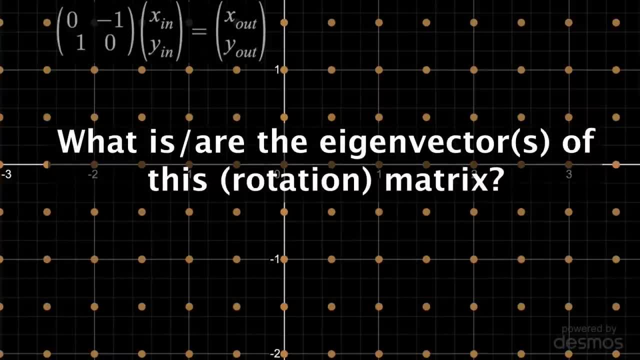 So the question is: what is the eigenvector of this new matrix? And, by the way, 0, 0 doesn't count. Well, considering an eigenvector is a vector not rotated by the matrix. we can say that. 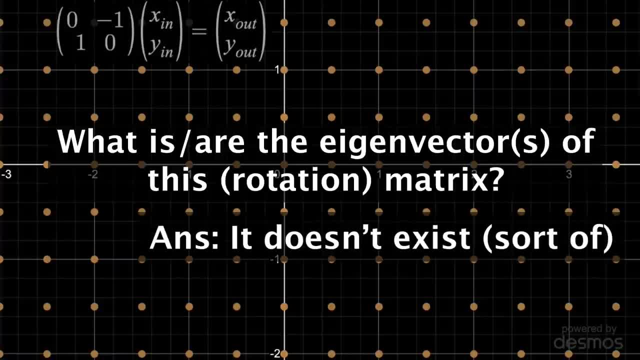 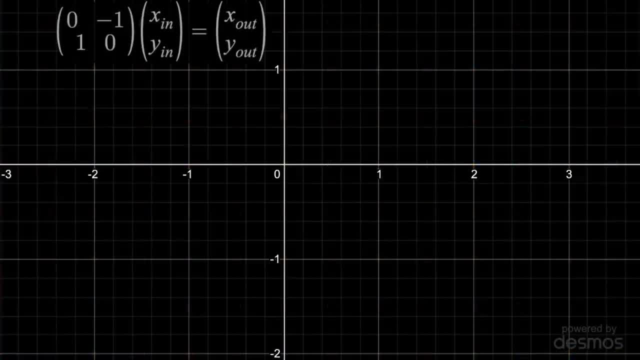 an eigenvector doesn't exist here, because every vector besides 0, 0 gets rotated. When you go through with the analysis, though, you do come out with eigenvectors and eigenvalues. However, they're imaginary. They're not real. 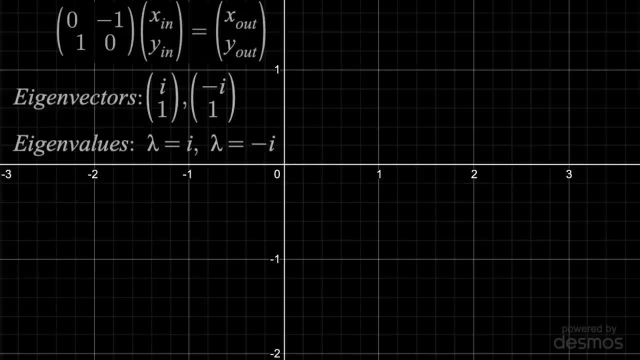 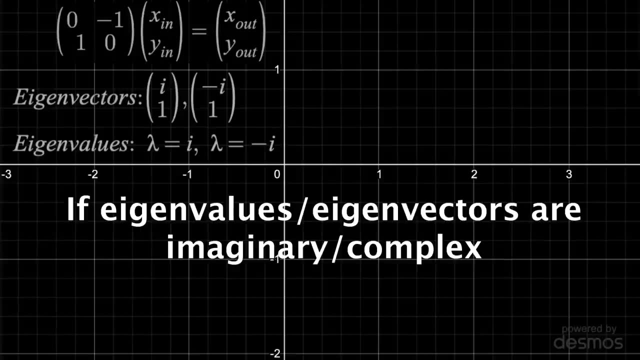 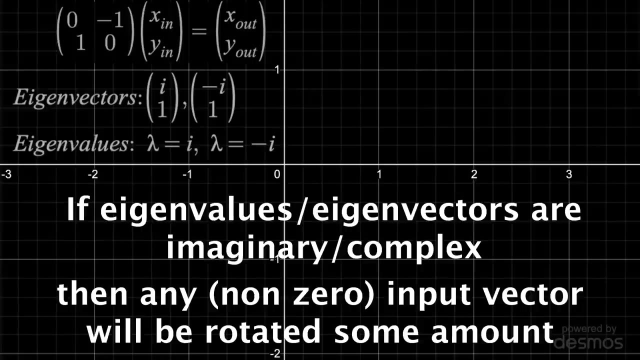 They're imaginary. much visual intuition behind this. what we care about is this simple fact: if the eigenvalue slash vectors are imaginary or just have an imaginary component, then any nonzero real input vector will be rotated by some amount from the matrix multiplication. it may be scaled, it may not, but some rotation will definitely. 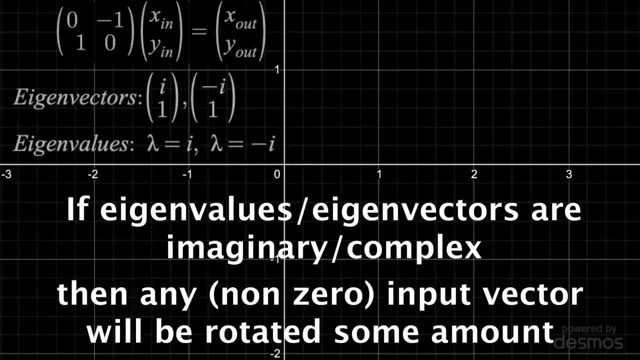 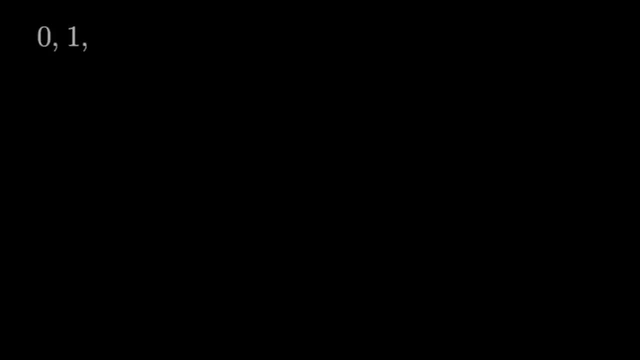 occur now. the first visual application we're going to see the eigenvectors and eigenvalues is the Fibonacci sequence. as most of you know, this is the sequence that starts with 0, then 1, and you just add those to get the next term, then you. 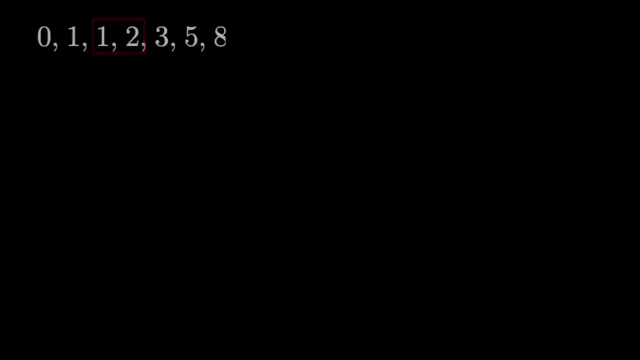 add these to get the next, and this continues so mathematically to get some term, you add the previous two. now, if I told you this number is part of that sequence, and ask for the next number, there's a nice visual way to find it without just going through the sequence itself. the reason for this visualization: 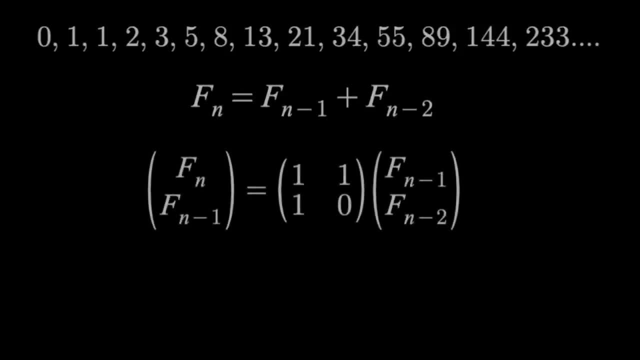 is because we can express the equation through matrix multiplication, just by a matrix multiplication. we can express the equation through matrix multiplication rules. you'll see: the first dot product gives us F? n minus 1 plus F? n minus 2 equals F? n. the same equation as above. the second dot product is trivial and 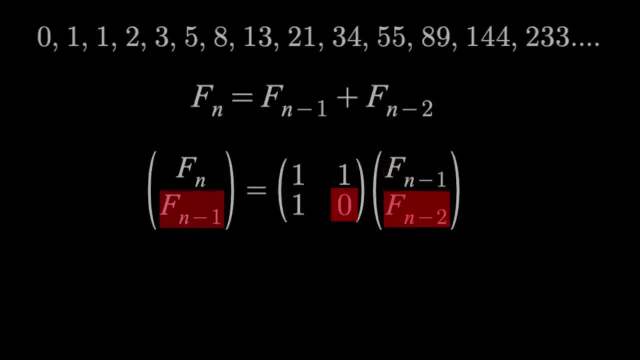 just says F n minus 1 plus 0 is itself. we just need this included so we can have a square matrix. so if I input any two neighboring terms like 8 and 5, the resulting output should just be the next term in the sequence, or 13 and the same. 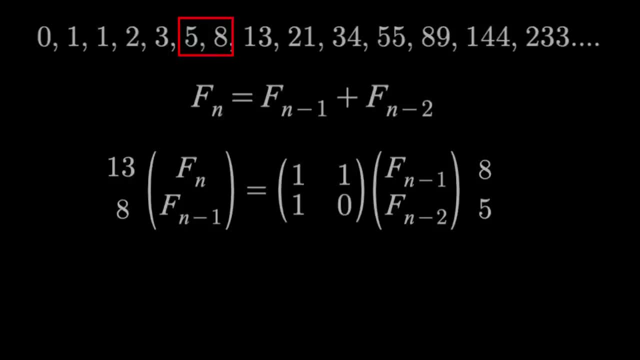 F, n minus 1 we input, or 8. essentially that's what we're going to see in this example. so we can see that the output is just the rectangle slid over by 1, and every matrix multiplication slides it over by 1 again. graphically, this says: if 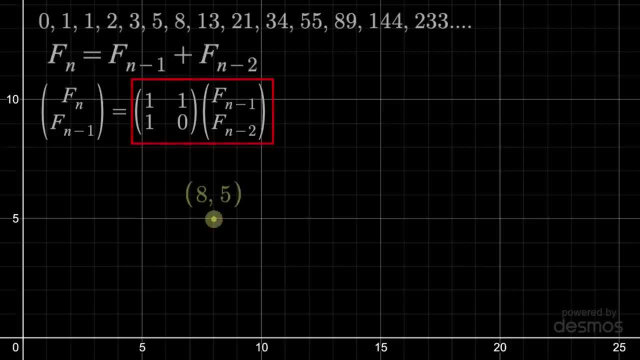 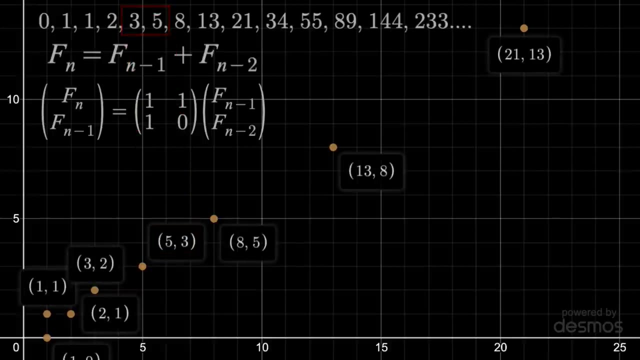 I have the vector 8 comma 5, then the matrix transformation should send it to 13 comma 8, which it does. but let me do that same transformation to several Fibonacci coordinates where any points or vectors represent two neighboring terms. if I keep a copy of the inputs then we can see the outputs just land on. 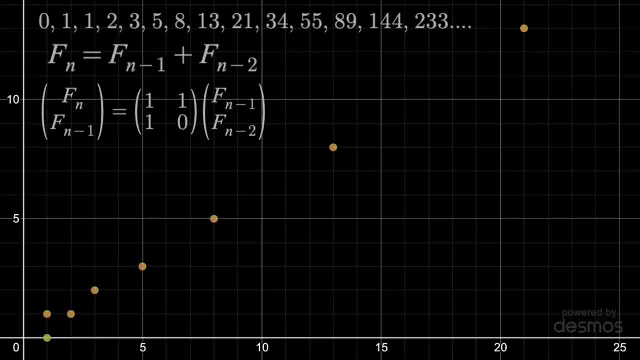 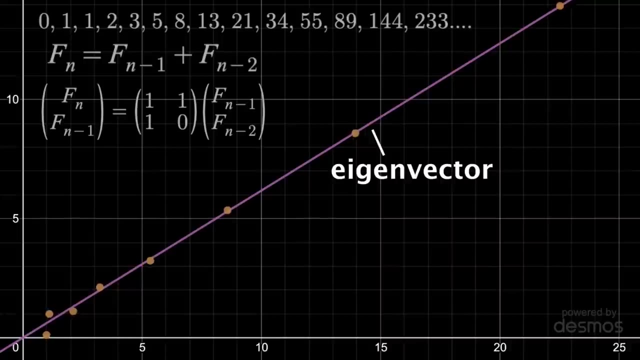 the next vector in the sequence. what we care about most, though, is the fact that these points all seem to be very close to this line here, because that is an eigenvector of our matrix. points really close to that line pretty much just move further up. there's mostly no rotation. the associated eigenvalue is actually: 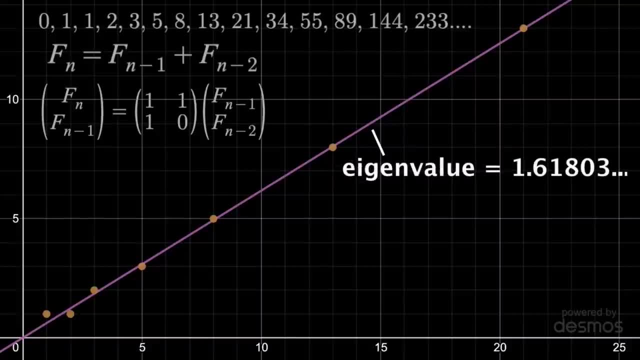 the golden ratio, or 1 plus root, 5 over 2. that's how much further the points get from the origin with each multiplication, roughly, since the points here aren't exactly on that line. this does make it easy to predict future terms, though, because even way further into the 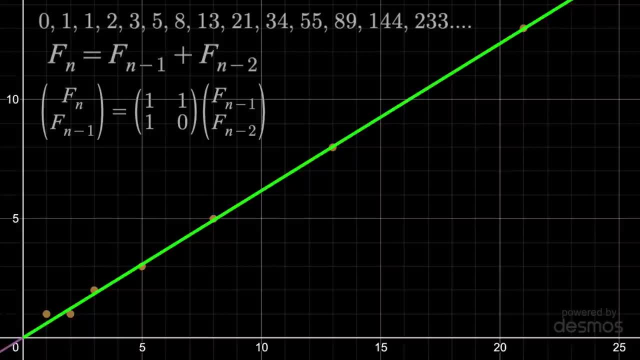 sequence, the coordinates will pretty much lie on this line. it's the eigen vector. those points aren't getting rotated off of it. so if I take any point and multiply its coordinates by the golden ratio, we get roughly the next point up. even for the early terms like this, the error is fairly small. but as we 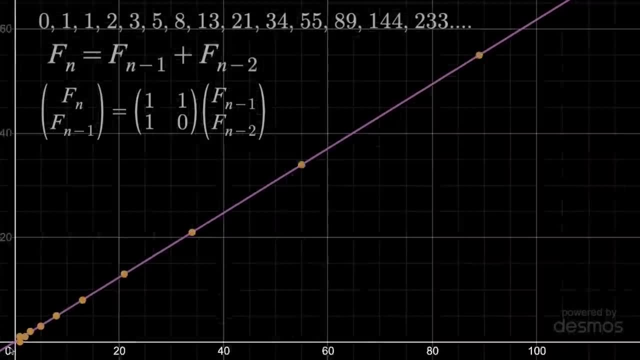 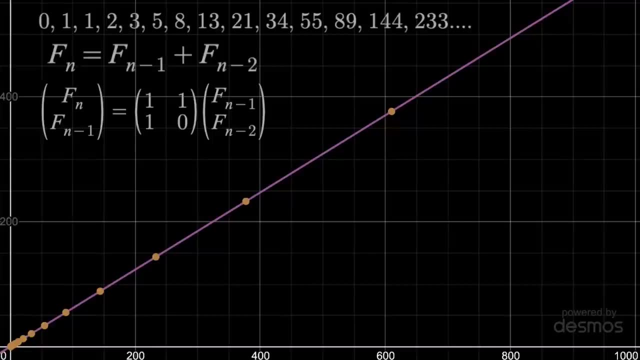 zoom out and let the term number go to infinity, it's pretty easy to get the error to zero and, as you can see, the points start to get extremely close to that eigenvector. this means, if I gave you some number way further up the sequence and ask for the next, you just multiply by the golden ratio and you: 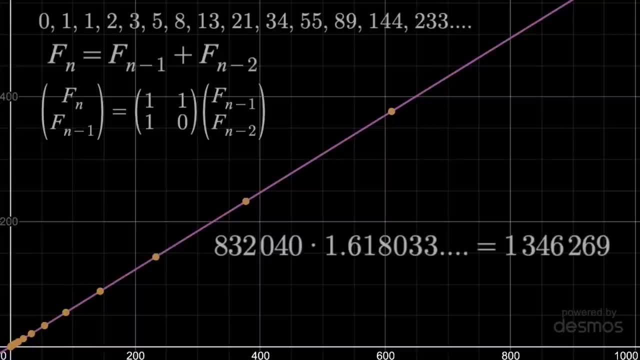 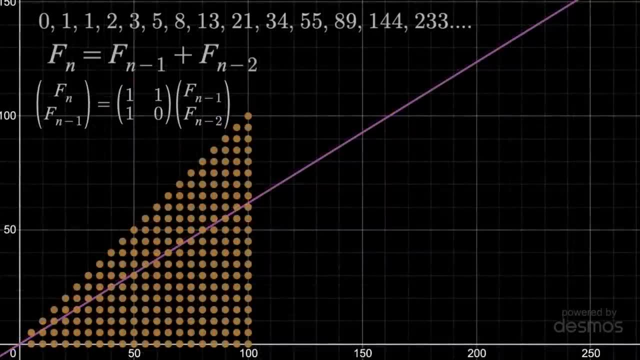 will find it to nearly exact precision. what I also find really interesting, though, is what happens when we apply that same matrix transformation to a bunch of random points. think of each of these as the first two numbers in a new Fibonacci sequence, with the same arithmetic but a different beginning. if 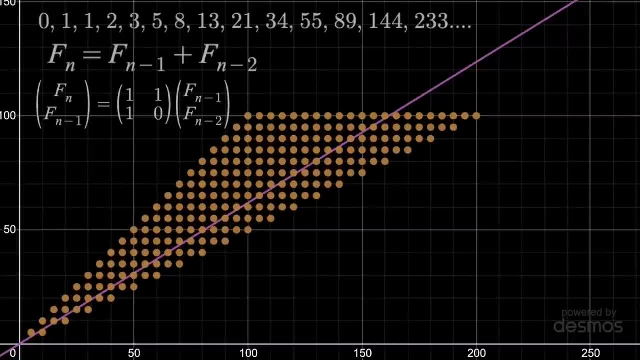 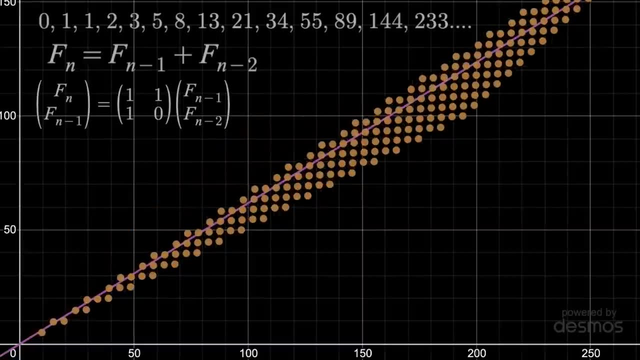 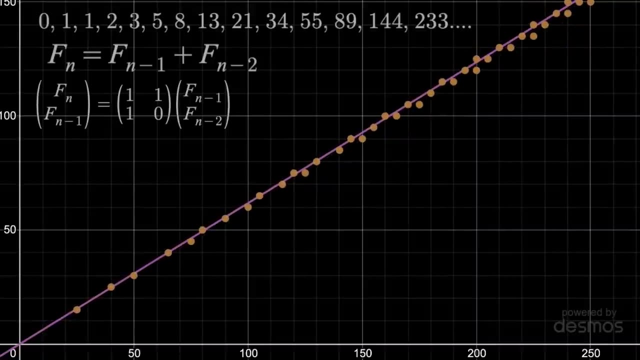 I apply the matrix multiplication, we get these points representing the second pair of numbers in the sequence. then another transformation gets us this set and as we keep going the points all get closer and closer to the eigenvector, meaning they all start to become scaled by the golden ratio. here I'll zoom out a. 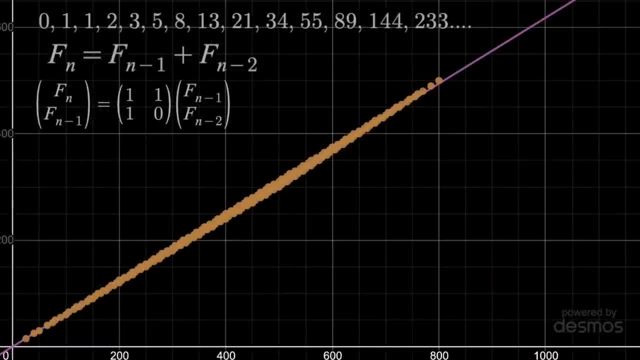 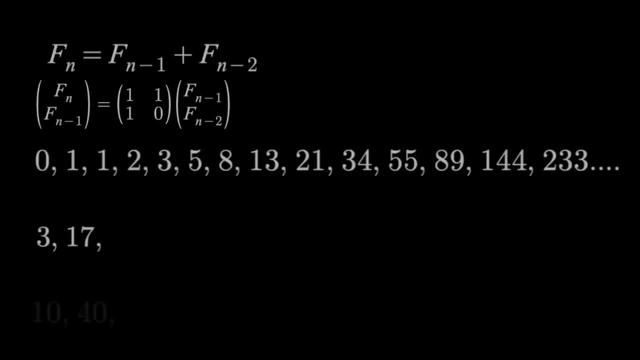 bit so you can see where they're at just after four multiplications. mathematically this tells us whether we multiply by the golden ratio or not. so we start by start at 0 and 1 or 3 and 17 or any other two positive numbers, so long as we use the same. 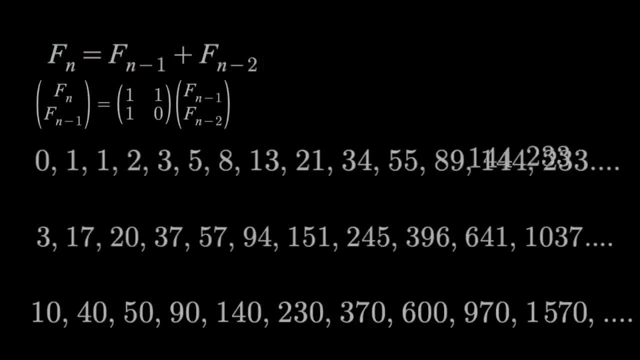 formula and add the two previous terms to get the next. the numbers will eventually just become a golden ratio, multiple of the previous. that ratio is built into the arithmetic and also this matrix and its eigenvalues, not the starting terms themselves. now for the people who want a more. 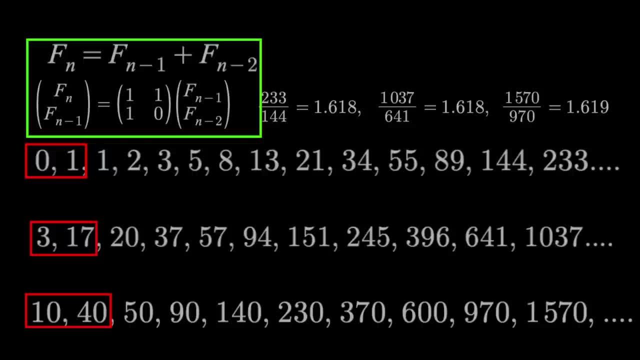 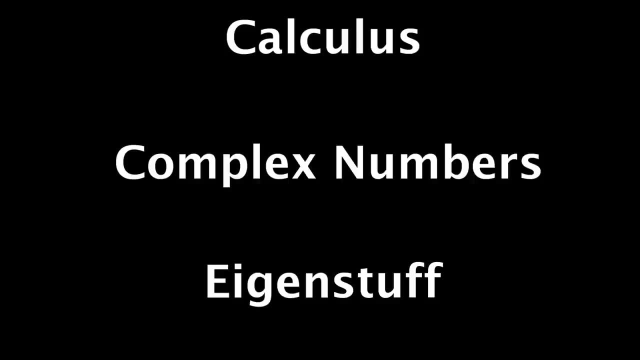 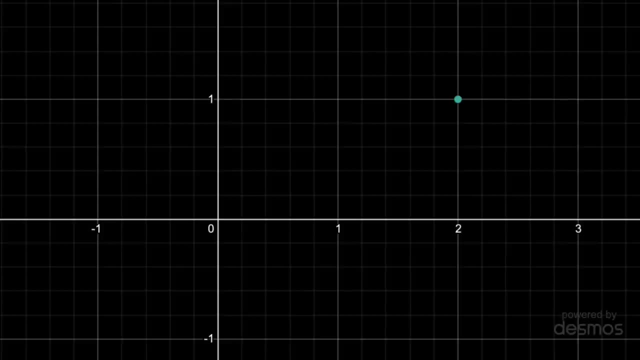 real world application. this next example is for you because it combines calculus with complex numbers, with eigen stuff real quick. we first have to answer a few questions, though. let's say i put a point randomly on the xy plane and tell you it will move as some function of time. my first: 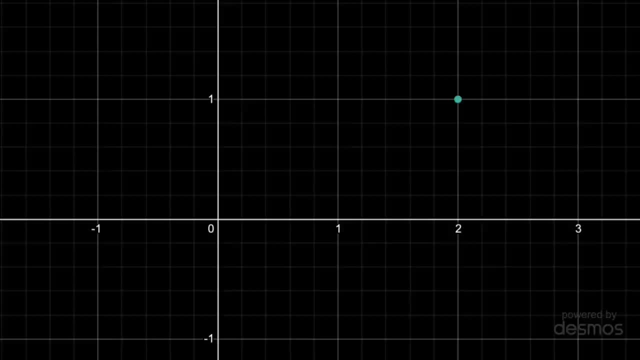 question is what values of dx dt and dy dt will cause it to move to the right. well, if you've taken calculus, this is pretty easy. dx dt has to be positive, while d y dt has to be positive. that'll cause a positive change in x, but no change in y, which is exactly what we want. 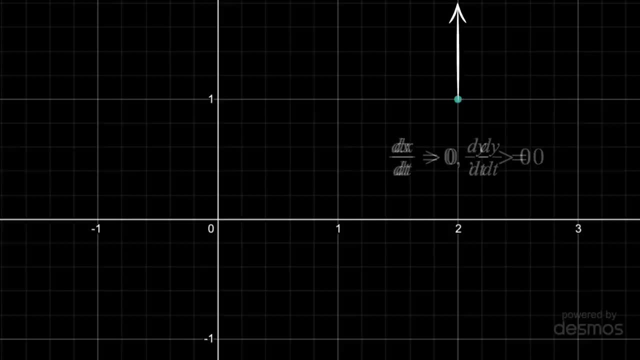 if i want the particle to move up, then d y dt has to be positive, while dx dt is zero. and you get the idea. but the slightly harder question is what if i want to move towards or away from the origin? well, in this case dy dt has to be one half of dx dt. we can see this if we think about. 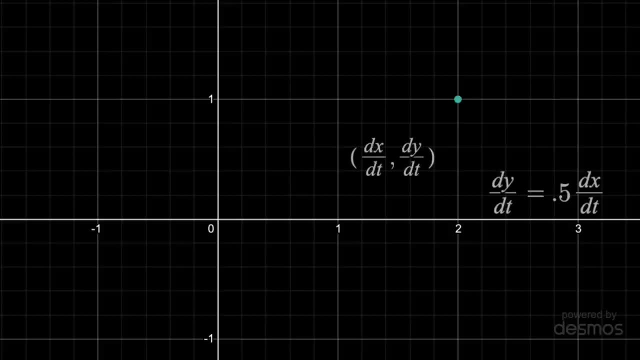 those two velocities as a coordinate, because dy dt will be half of dx dt and that's the same line that passes through the particle itself and the origin. the equation for this is: y equals one half x. just to show the visuals, if dx dt is 1 and dy dt is 0.5, like: 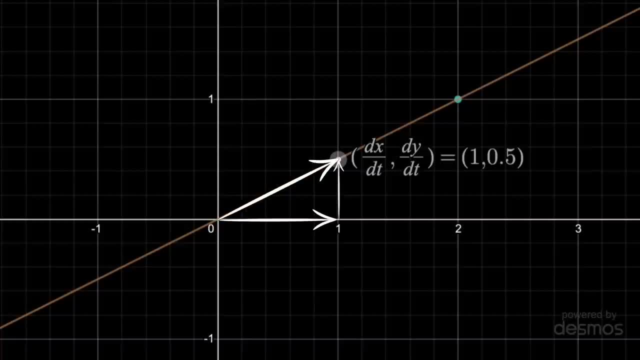 this coordinate shows, then the vector sum yields this here, which points directly away from the origin, and that's the direction the particle would move. any of these values will give us the same thing, though, while negative velocities will result in motion towards the origin. this will be the final answer in the following у equation: 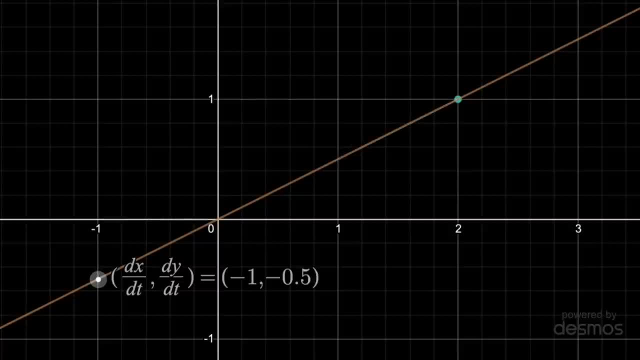 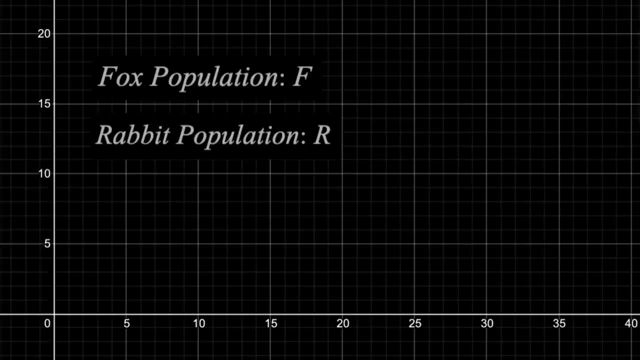 so we know the vector is one half of dx, dt, and that's the first value that we get, which is the origin of the origin of the element in the product. here's some of the explanations of this function. okay, now we're ready for the applications. let's say there's some population of foxes- we'll label f- and a population of rabbits- we'll label r. 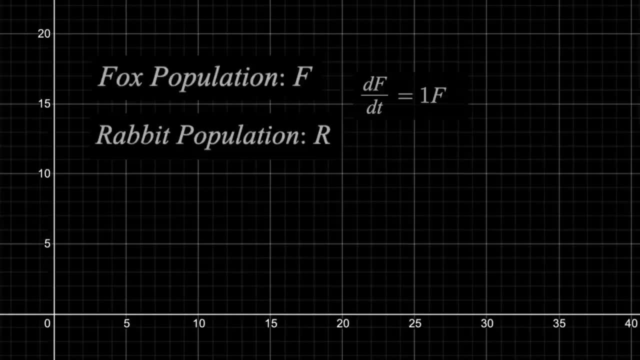 these variables will represent the number of each of those animals at any given time. then let's say that the population of foxes changes at a rate equal to its current population, upper bound on population, because it will simplify things. If you've completed calc 1, you know this. 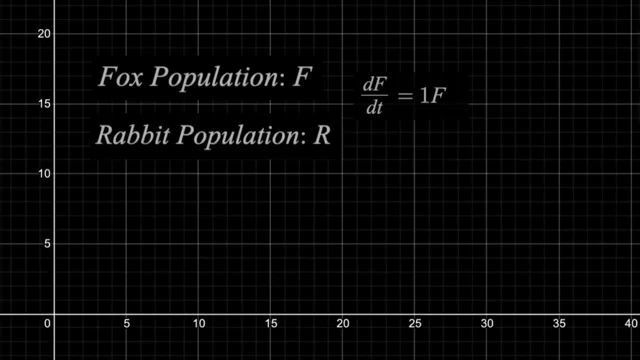 leads to exponential growth. Now the population of rabbits will grow at a rate three times their current population, much faster than the foxes. However, they will die or be eaten at a rate equal to how many foxes there are. This makes things more difficult, but overall, the goal is to see. 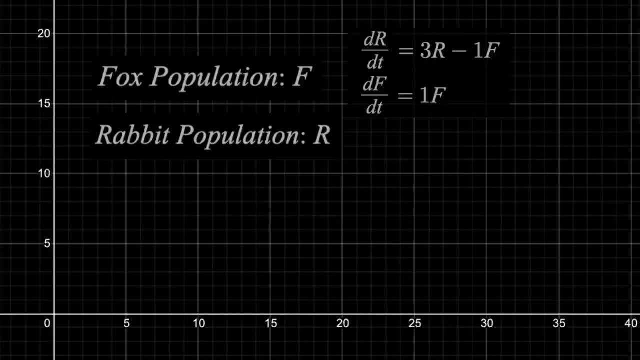 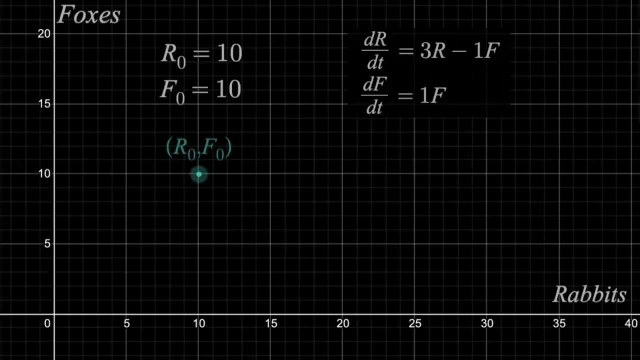 what will happen over time if we start with some arbitrary number of both animals. Now, graphically, just consider the x-axis to be rabbit population at any time and the y-axis will be foxes. If we say there are initially 10 rabbits and 10 foxes, that's represented as a point at 10,10.. If we plug, 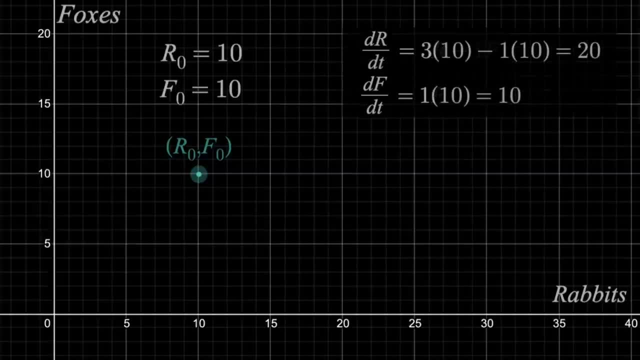 those numbers into the equations, then we get out the derivatives, which tells us the rabbits will be increasing at twice the rate as the foxes just at that time. This is just like before. so if we put the dr dt and the df dt component at that point, basically like velocities, 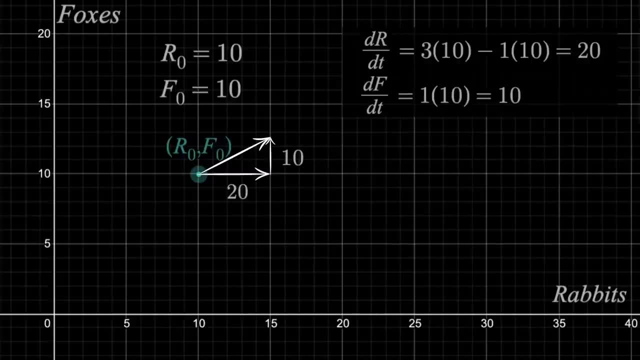 the vector sum will tell us that it will move up and to the right just at that moment. This just means both the populations are increasing, because even though the rabbits are being eaten, they're reproducing fast enough to increase in population. Don't worry about the length of the vector, though. 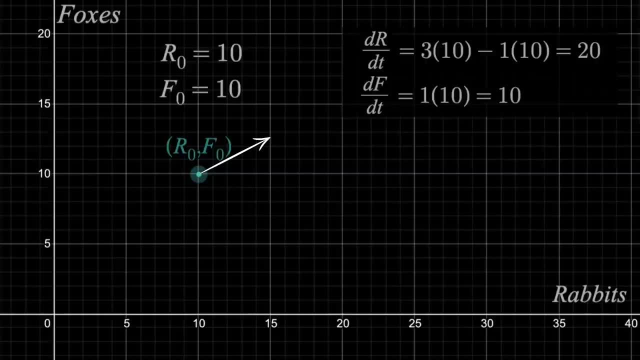 just the direction Now. had the rabbit population start at two instead. then plugging those into the equations tells us that the rabbits will decrease in number. Essentially. there's not enough of them now and they'll die out faster than they can reach. So if we plug those into the equations, 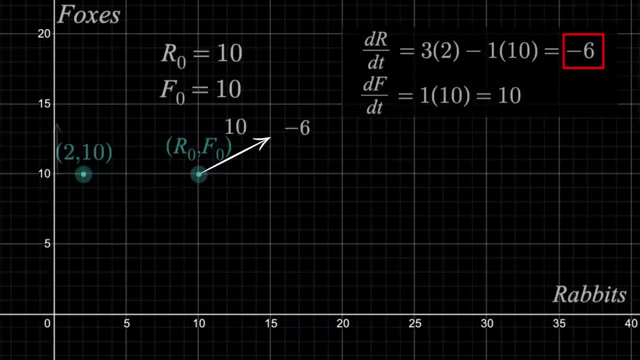 we can see that the rabbits are going to reproduce. So plotting those vector components tells us that at that instant the point will move up and to the left. It looks like we're headed towards zero rabbits. If I did this for every point, we'd make kind of like a slope field, but it's really called a phase. 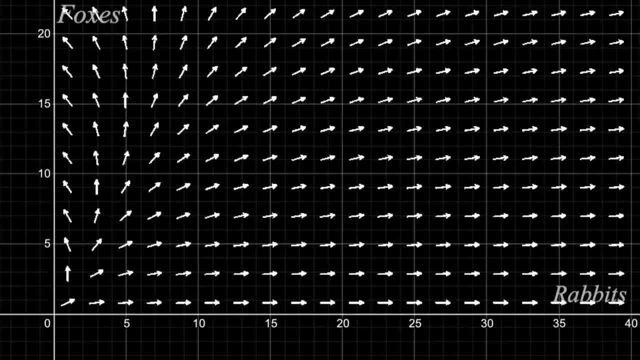 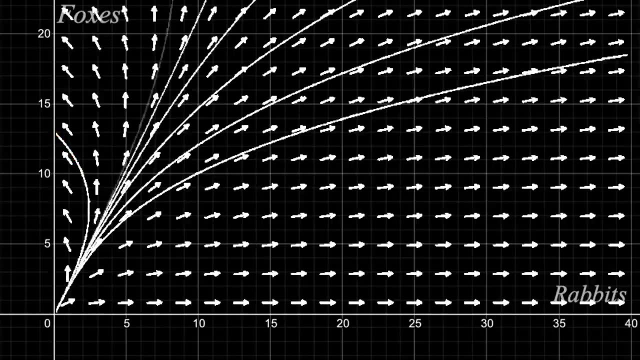 plane for a system of differential equations. If I start at, let's say, 10,10,, we just fold the arrows and see how the population will change over time. Starting at 2,10,, we see that it eventually does. and these would just be a bunch of other scenarios, depending on where you start. 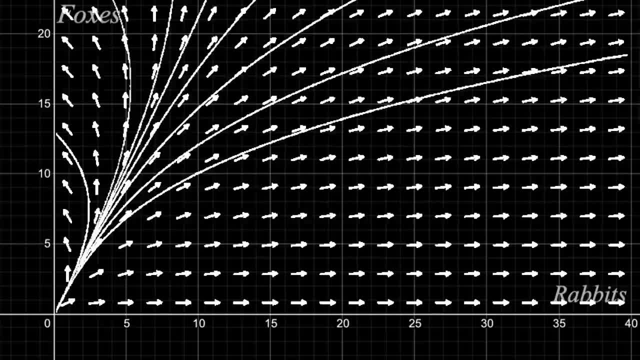 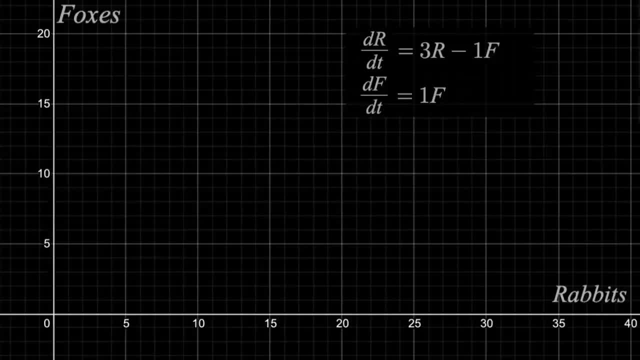 What you're seeing are the solutions to that set of differential equations for different initial conditions. But making a phase plane one point at a time is way too tedious, so let's look at this another way. I'm going to take the coefficients and put them into a matrix that'll 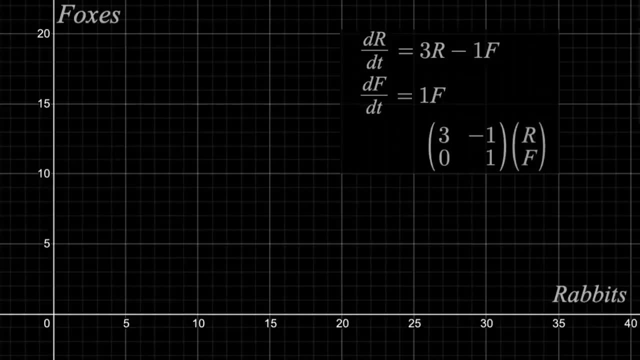 be multiplied by the two variables r and f. I'll call the derivatives just r prime and f prime and by matrix multiplication. you'll see these are the same thing. Now we can apply matrix transformations from before, but this time notice that the inputs 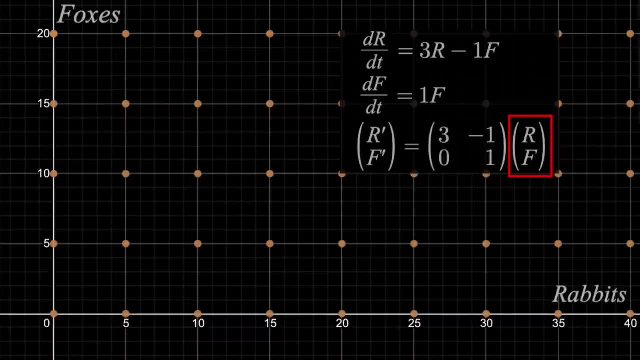 are the rabbit and fox populations. Those are the points you're seeing. However, applying the matrix multiplication will output velocities in a way, or rates of change of the population, not new ones. Here I'll put 10,10 in a different color and do the multiplication while keeping a copy of it at 10,10.. 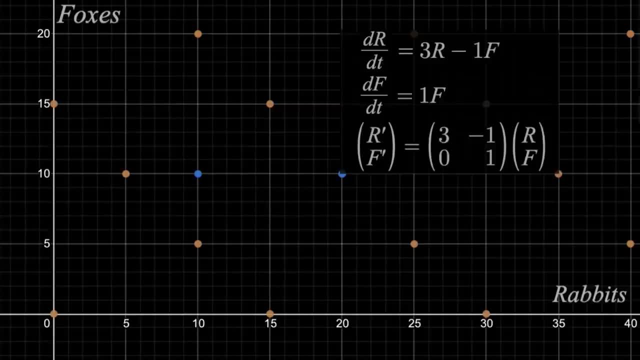 Here we have the outputs, but again these represent the simultaneous rates of change for their associated inputs. As in: at 10,10 we'd have an r prime of 20 and f prime of 10.. If I proportionally shrink these and put them on top of the input, then this tells: 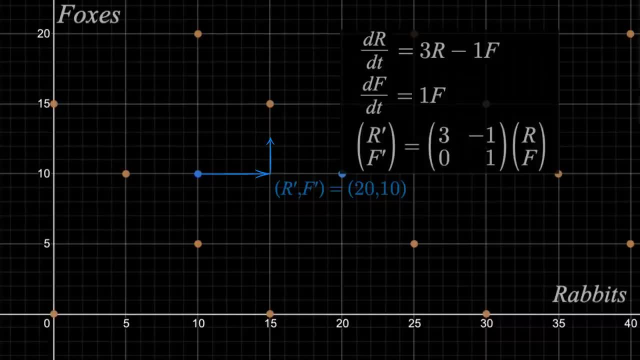 us exactly what we saw before, That if you put 10 rabbits and 10 foxes in our simulation and hit play at that moment, both populations would increase, but rabbits would be increasing twice as fast. Moving vector though: If I rewind you'll find anything on this line, or the x-axis is not rotated. 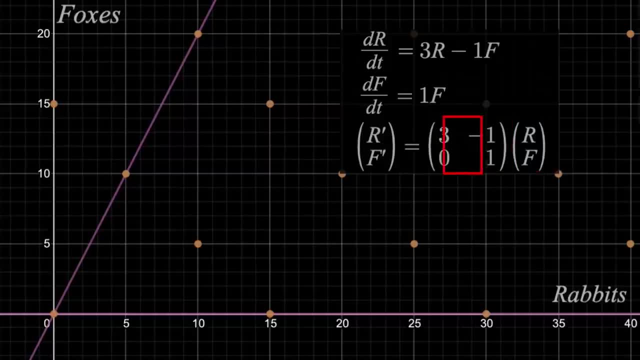 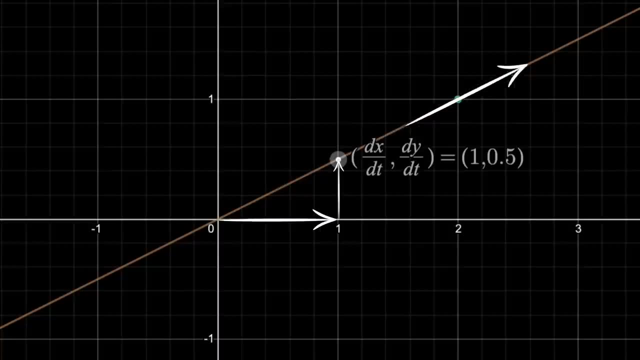 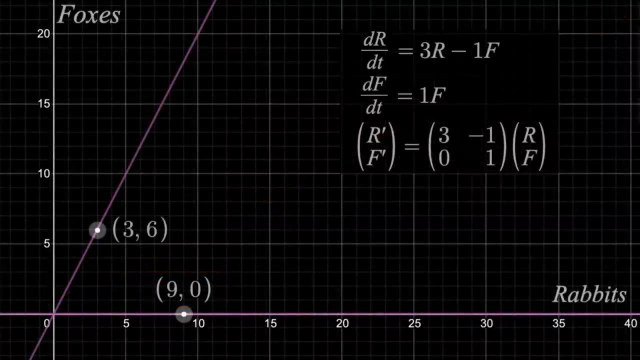 This means any inputs on those lines will also have velocity values on those lines, And remember from before when that was the case, it meant motion would be along that line. This means if we have nine rabbits and zero foxes, or let's say three rabbits and six foxes, as long as we're 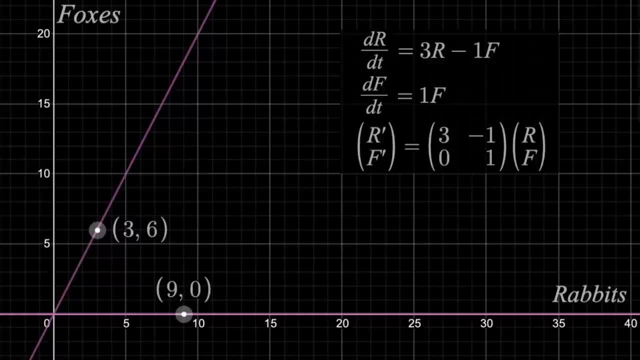 using eigenvectors and let the simulation run. the population values will stay on those lines forever. See, the bottom eigenvector is obvious. If you start with only rabbits, then after some time you'll have more rabbits, no surprise. But the top one is kind of like a sweet spot. 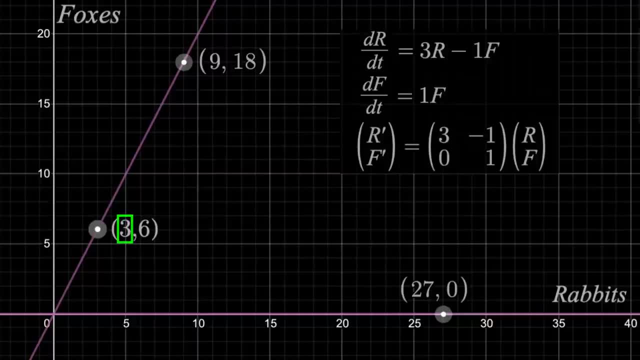 where you start with twice as many foxes as rabbits and over time that ratio never changes. There's just enough foxes where the rabbits don't take over in population, but not enough where the rabbits die out completely. Everything stays in proportion. 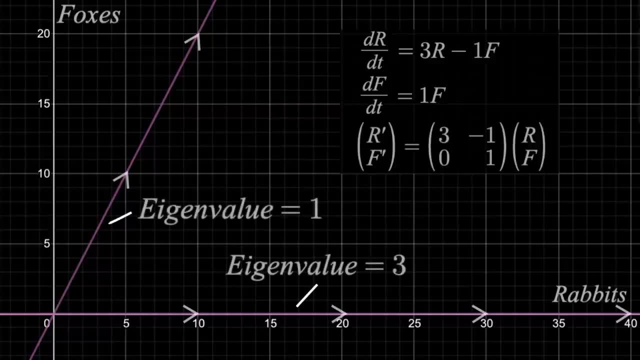 Both of these have positive eigenvalues, which is why the points move away from the origin and not towards it. But just these eigenvectors are enough for us to approximate the evolution of the system for any initial conditions, Because the flow from any other initial populations kind of follows the eigenvectors. 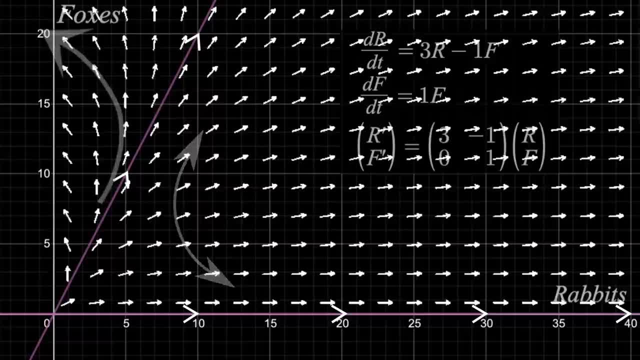 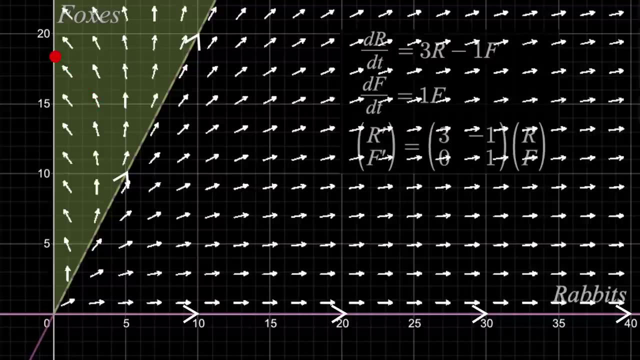 which is why the phase plane looked the way that it did. Plus, the top eigenvector divided this into interesting regions. The neighboring populations located above it will result in no rabbits. eventually, all these arrows led to the y-axis. This is where the foxes quote win. 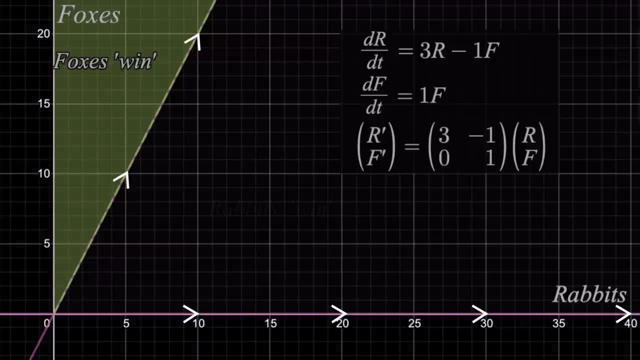 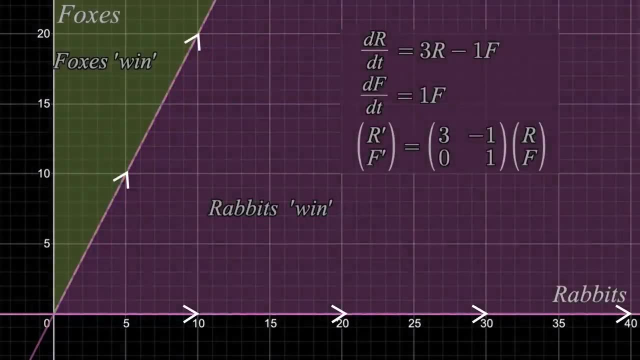 they kill off the rabbits faster than the rabbits can reproduce. But below that eigenvector and above the other is where the rabbits sort of win Really. it means over time they outpopulate the foxes more and more. They're still being eaten, but they are reproducing much faster. 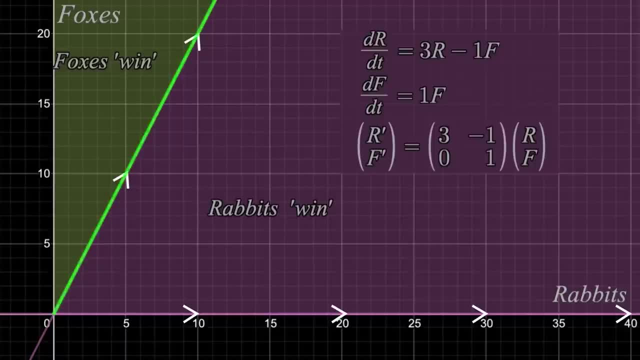 The eigenvector is a very strong force that's always going to be there and it's going to give the foxes a big boost. And the eigenvector is the order in which they can reproduce more rapidly again, the sweet spot where everything stays in proportion. This is why, before 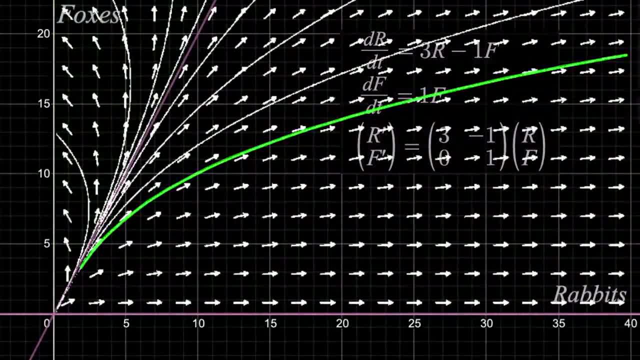 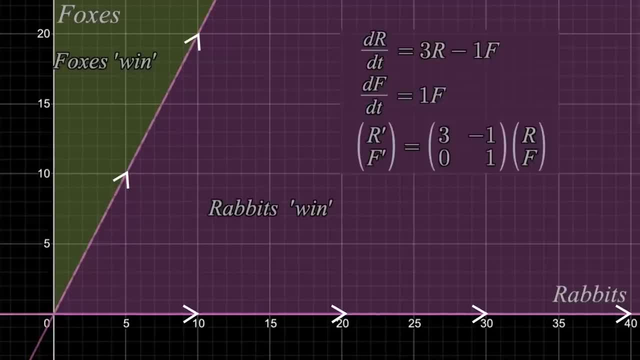 we saw some paths fly off to the right and others turn towards the left. It was all dependent on which side of the eigenvector we started on. And to add some dynamics here, you'll see if I increase this number and make it so. the 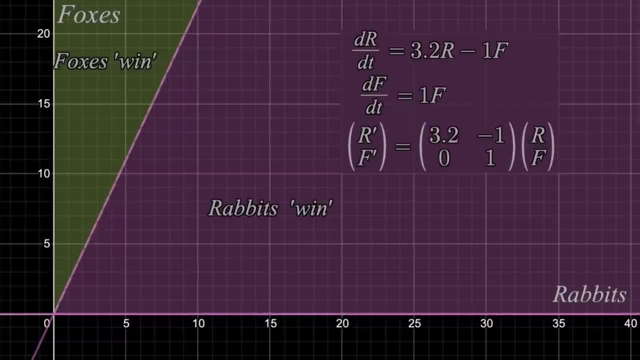 rabbits reproduce faster and the eigenvector moves up, increasing the rabbits win section as expected. If I make the foxes reproduce faster, then it goes back down, increasing that foxes win region. The most well-known use of this, though, is with masses on a spring, Because, instead of plotting animal 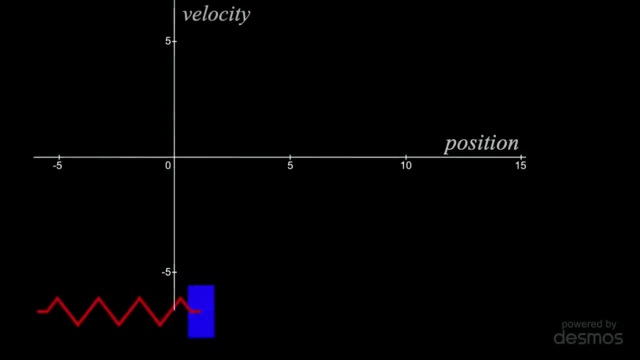 populations. we'll plot position versus velocity. If I pull the mass to the left but give it no initial velocity, that corresponds to this point on the graph. If I let go, assuming no damping, it will oscillate back and forth forever On the phase plane. this corresponds to circling. 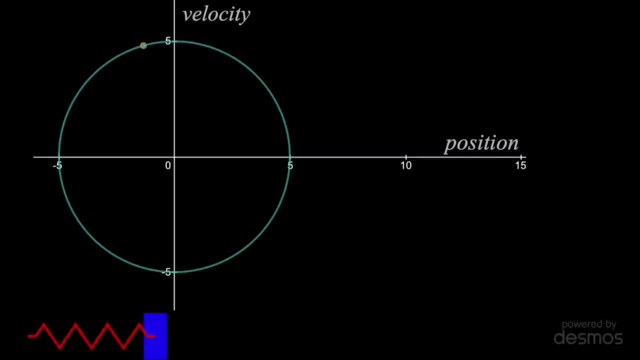 the origin between max displacement and no velocity to max velocity and no displacement, and so on forever. Now, the equation that represents this is MA or MV. prime equals negative KX minus BV, where K is the spring constant and B is the damping coefficient. Currently, the mass and spring constant are 1, while B is. 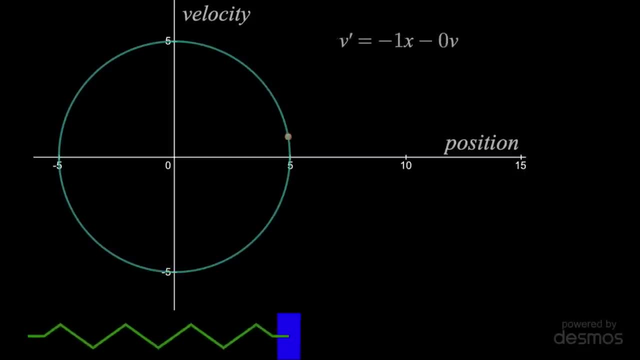 0. so this is the actual equation And, as you guys probably know, the derivative of position is velocity. Now, why am I writing things like this? Because, look, we have two derivatives, some coefficients and those same variables without the prime, just like before. It's the same type of problem which comes down to. 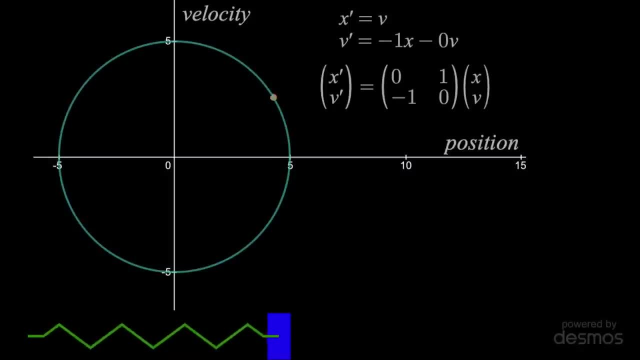 finding eigen things. However, in this case, the eigenvalues are imaginary, thus so are the eigenvectors. Now, do you guys remember before when I said that imaginary eigenvalues correspond to rotation? Well, here it is again in a much more visual way, For these systems of differential equations purely imaginary. 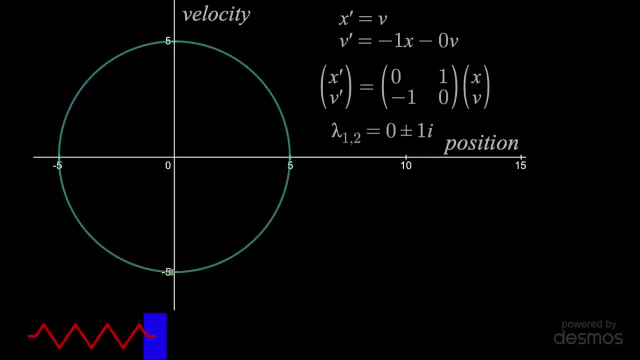 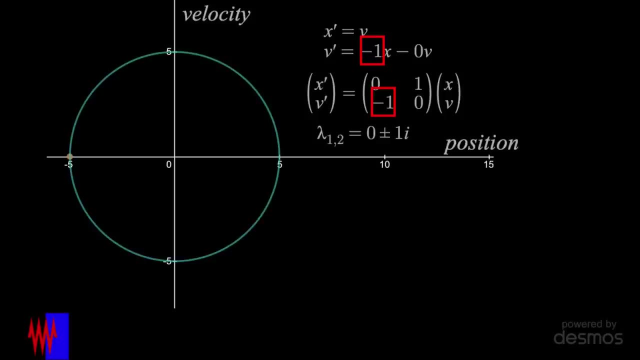 values mean only rotation, no decay to equilibrium or diverging away from it. Now, if I increase the spring constant and make the spring stronger, we still expect no decay. but there should be some higher velocities. So watch what happens as I increment it. Now we get more of an oval shape, showing that the max velocity has. 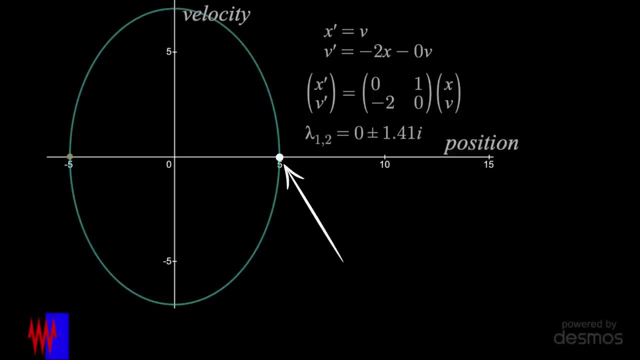 increased, but the max position does not, since it starts from the same point. The eigenvalue is still imaginary though, meaning only rotation and no decay. If we add some light damping, like put the block in some fluid, we expect the block to oscillate, but decay to equilibrium in the process. So first watch what happens. 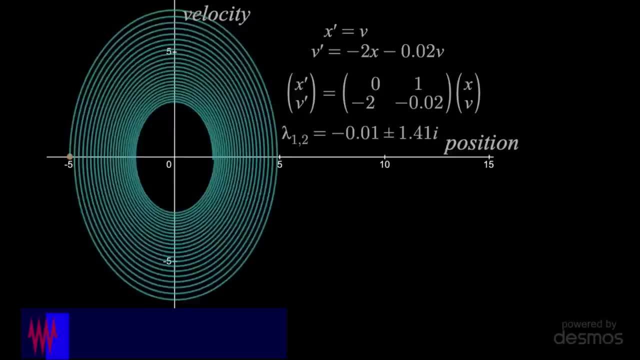 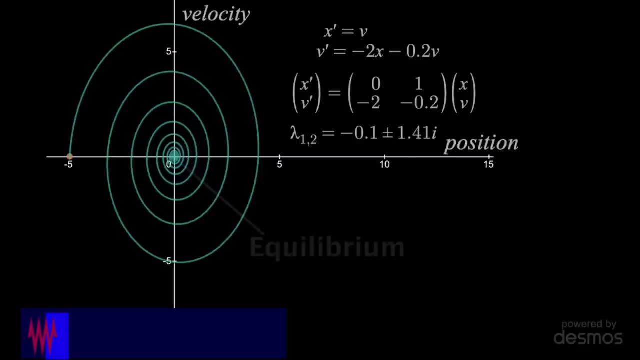 to the phase plane. as I change that damping coefficient, You'll see it now- spirals into the origin, aka the equilibrium, where there's no velocity or displacement, Which matches what we expect with the decay that comes from the damping, From the eigenvalue perspective, we gain even more intuition because, on top of imaginary 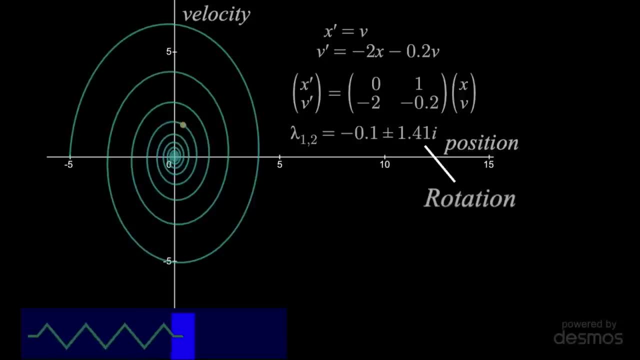 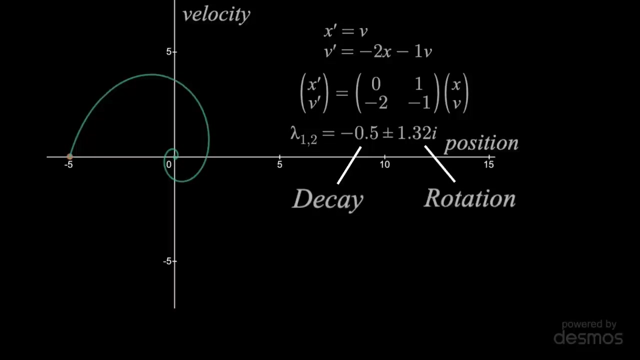 components corresponding to rotation. we can now see that negative real components correspond to decay. As in, the system is stable and will go to equilibrium eventually. Here I'll increase the damping coefficient even more where we see faster decay on the phase plane and, as expected, a more negative real component of our eigenvalue. And if it were possible to have a 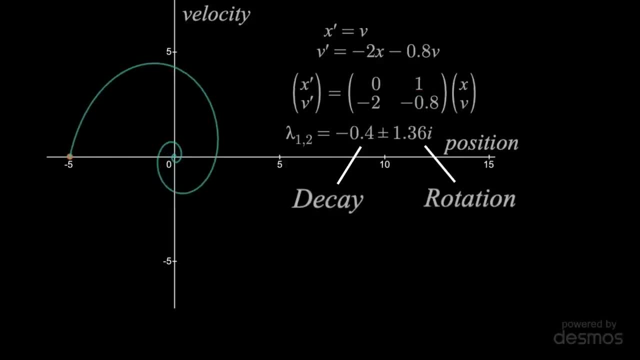 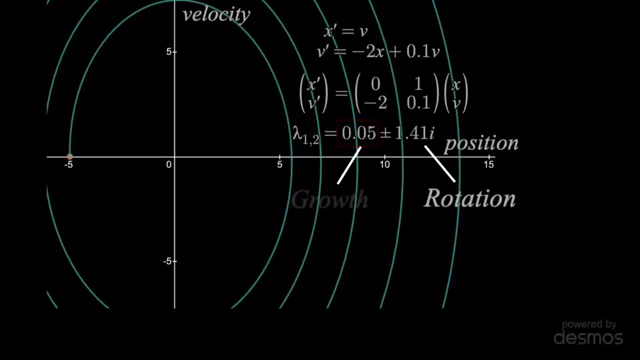 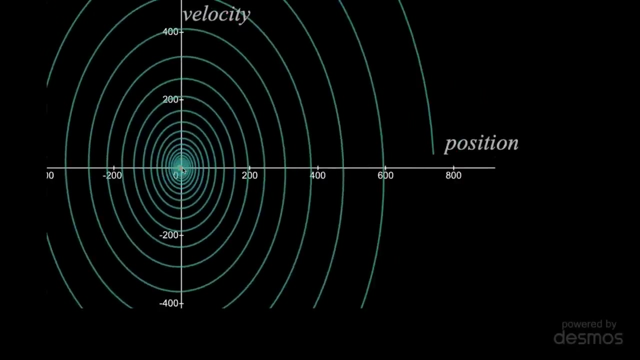 positive damping coefficient here, which I'll change it to, Then that gives us a positive real component which corresponds to growth or instability, And this really means that the phase plane will spiral away from equilibrium. Now, so far we've seen how eigenvalues and eigenvectors 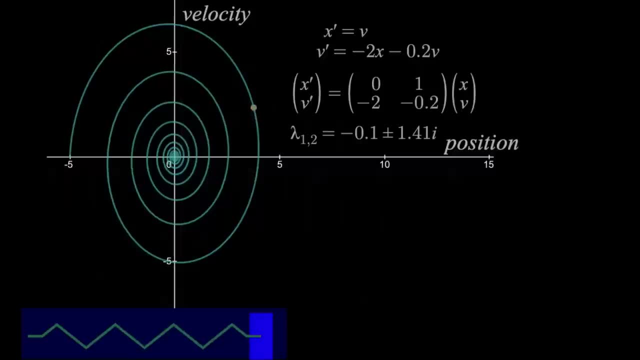 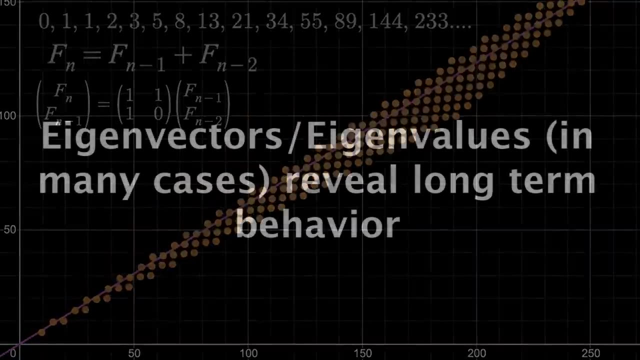 can give us a real visual sense for what can happen to a system or a sequence after a long time or many iterations. This isn't always the case, but in many situations eigenvectors and eigenvalues reveal that long-term behavior. That's one reason why 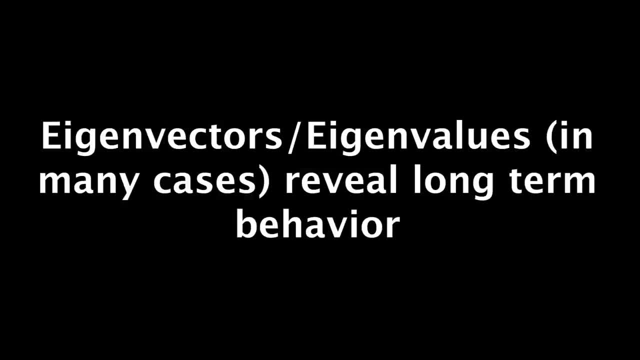 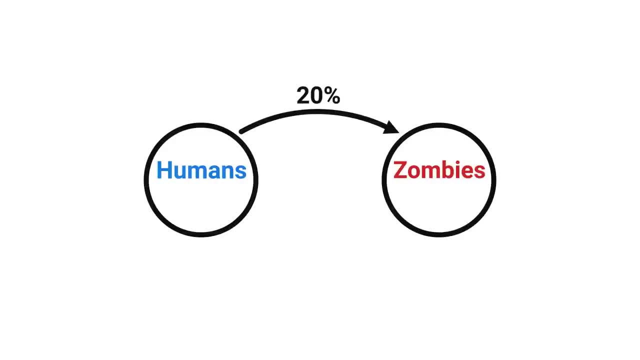 they're so useful In the applications of matrices video. I showed an example of this with a zombie apocalypse scenario, Where, in a quarantine area, every hour some percentage of humans turn into zombies, but there is a cure that converts a percentage of zombies back to humans, Since 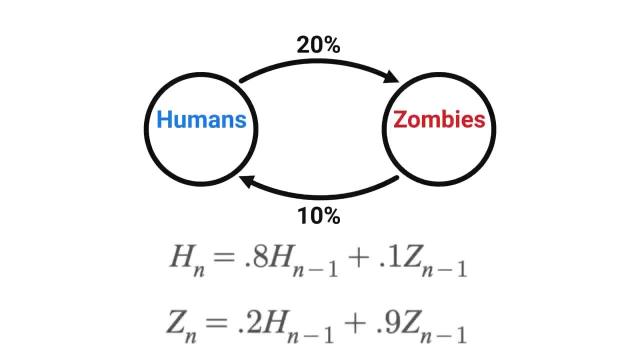 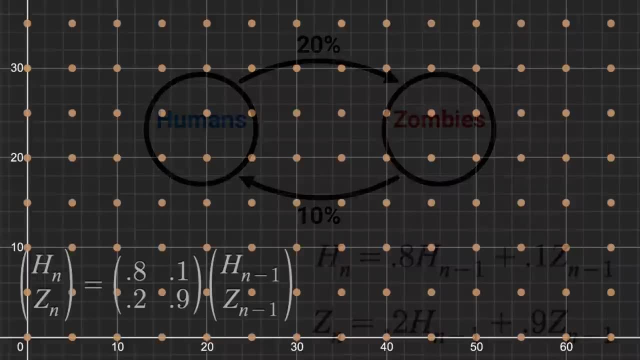 the new population of humans and zombies after each hour can be calculated with linear equations. we can change it into a matrix problem to see what happens in the long run. If I use Desmos instead, we can see, with several starting points representing initial populations of humans and zombies, the 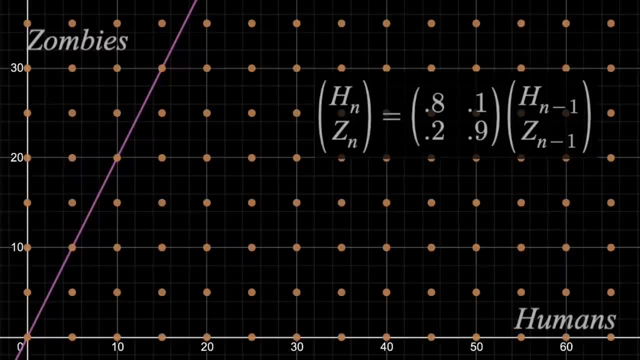 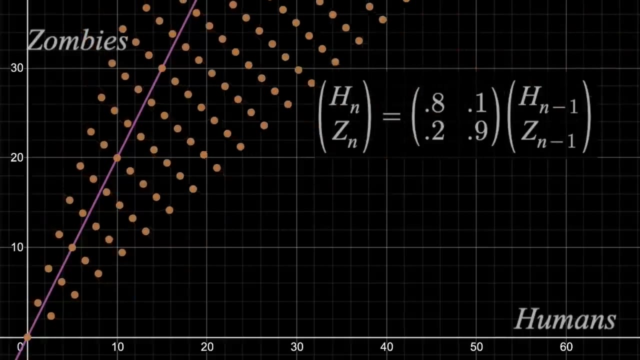 eigenvector reveals the equilibrium of the system, And since the eigenvalue is one, once the populations are on that, then they won't change, But everything else will move towards it with each hour. So, after many iterations, the system will converge to a point where there are twice as many zombies. 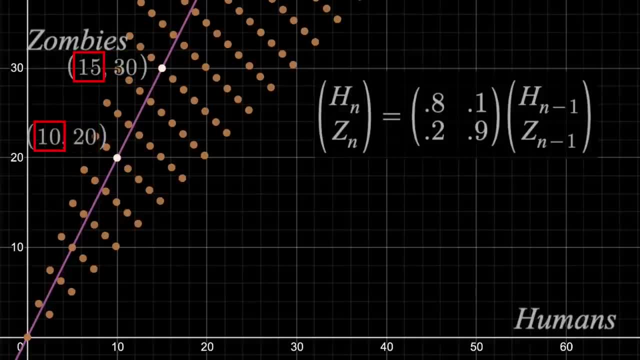 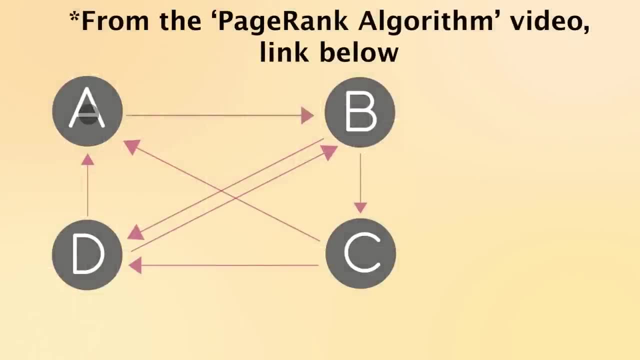 as humans And again it's the eigenvector that reveals that long-term behavior. Or let's say we had several nodes and one way past connecting them. If you were to just randomly walk this network all day and wanted to know how much time you'd spend at each node, on average it becomes. 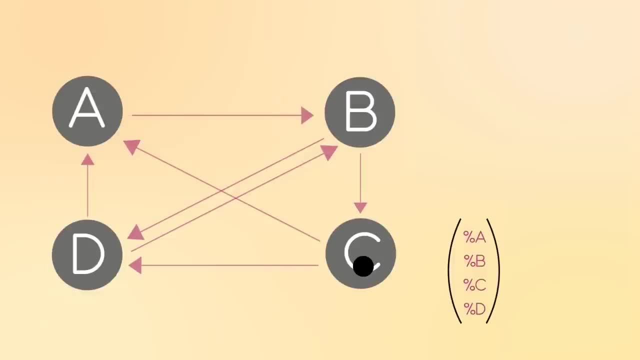 a matrix problem Because, since everything's random, we can write out the probabilities Like, if you're at A, there's a 100% chance of going to B, but once you're there, you have a 50% chance of going to C or D, and you just 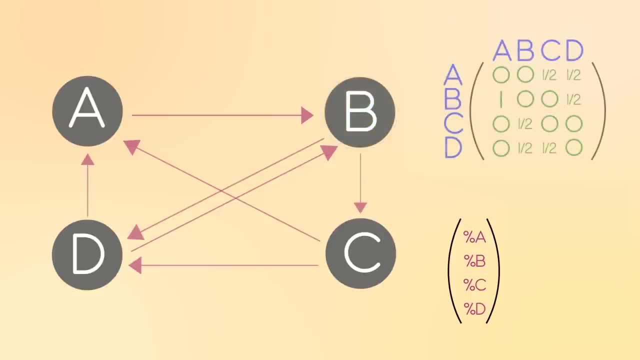 do this for every edge. If we put those probabilities into a matrix where you can see, like the chance of going from A to B is 100% but B to C is 50%, it turns out the eigenvector of that matrix reveals the percentage of time you'll spend at each node. If we instead think of those nodes as websites, 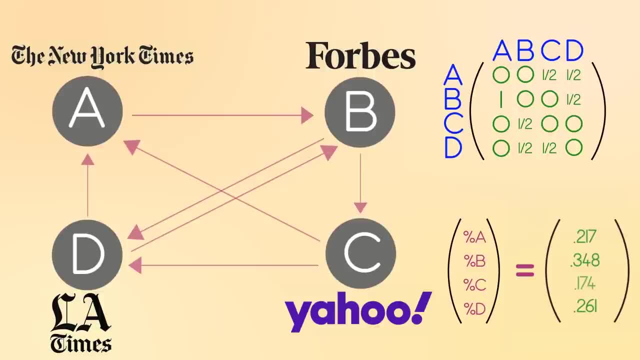 and the edges as links between them. then you get the basic idea of how Google ranks web pages. As in the beginning, the basic idea of Google page rank was determining which site you'd spend more time on if you randomly clicked links all day, And that ranking matrix is really just an eigenvector. 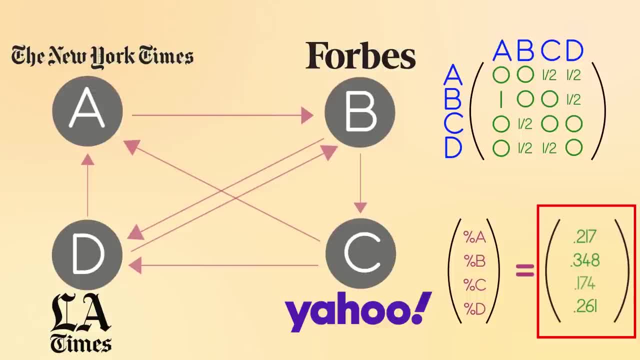 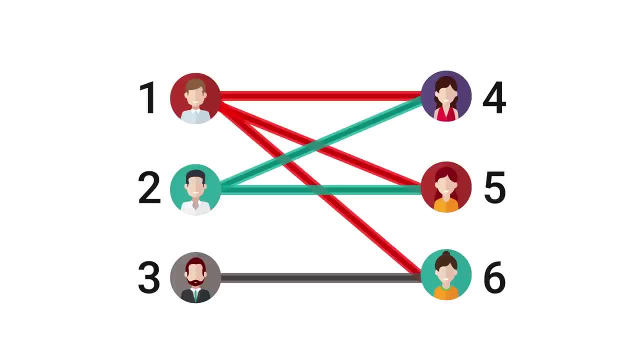 But it's not always about long-term behavior. For example, also from that previous video, I didn't mention something about the dating app network example. This was when three men, labeled one through three, and three women, four through six, were matched on a dating site, as shown. 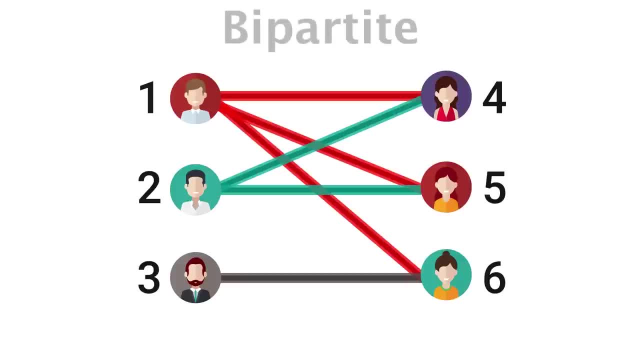 But there were no same-sex matches, which makes this a bipartite graph. Bipartite just means the network can be separated into two different sets such that each one of these has no internal connections. Now, when we made the adjacency matrix for this, where, if like person one 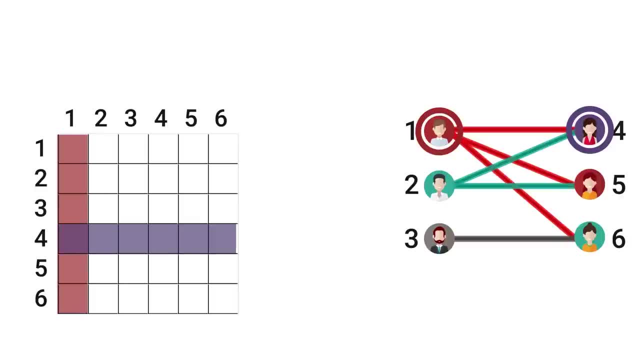 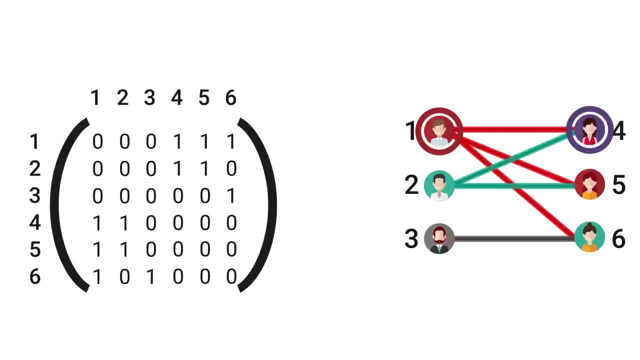 and four are connected, then we see a one in column one in row four as well as row one in column four, and if two people were not connected, there would be a zero giving us this. What I didn't say is that these were the eigenvalues. It turns out. if a graph is bipartite, then the eigenvalues of this. 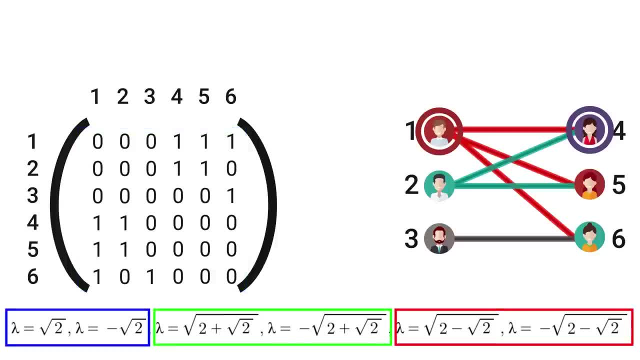 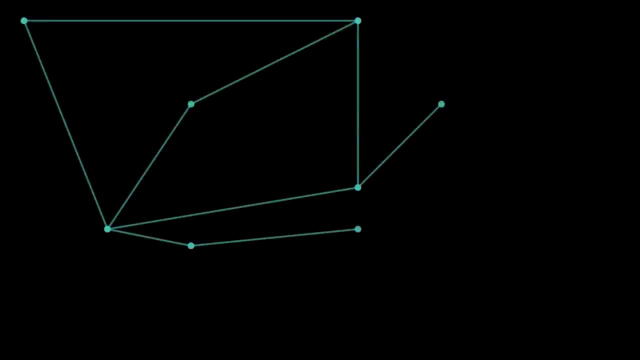 graph will come in plus and minus pairs. If we allowed a same-sex match, then this is no longer bipartite and the eigenvalues don't come in those pairs. So if I gave you a network like this, it's not obvious whether it's bipartite just by looking at it. But if I label the nodes and make an 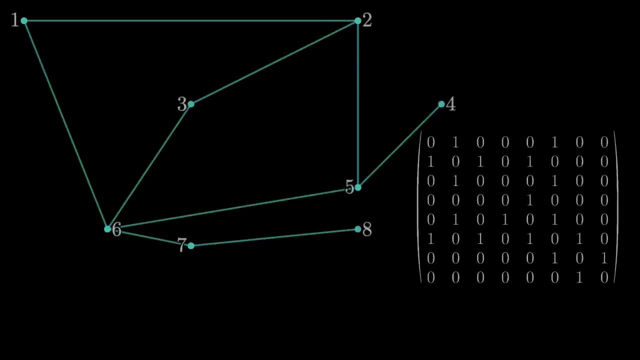 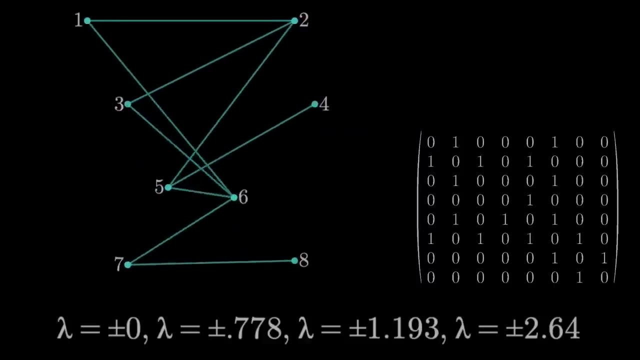 adjacency matrix. based on those connections, I find the eigenvalues all come in plus and minus pairs, which tells us, yes, the graph is bipartite, and if we rearrange, that becomes more obvious. Looking at how clustered a graph is also involves eigenvalue analysis, by the way, and this can reveal: 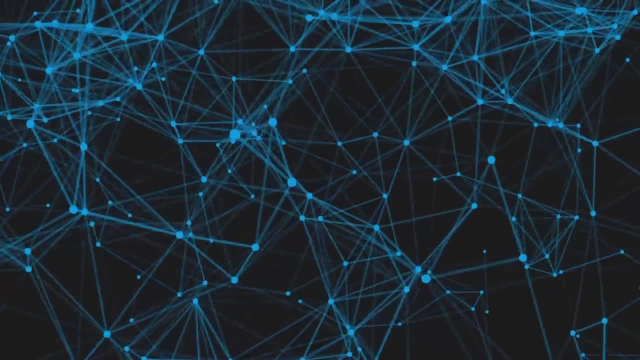 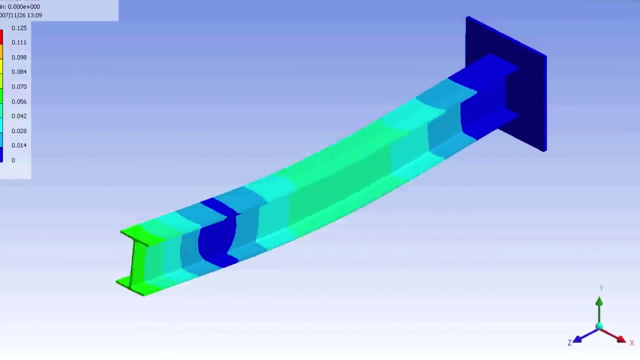 hidden patterns among very chaotic graphs. You can look up spectral clustering to learn more about this, though. Then eigenvalues show up in frequency analysis, as they're used to find the natural frequency of a system. Of course they appear in circuits due to the similarities between those. 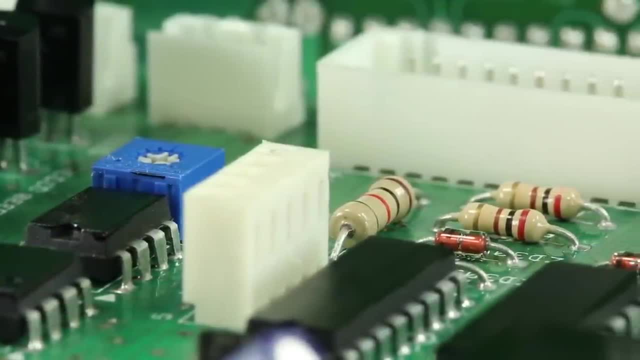 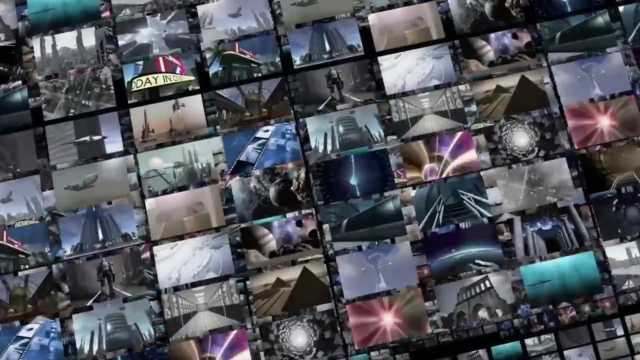 and masses on the spring. Eigenvalues can help us understand how quickly a disease will spread throughout a population. They're used in data compression and facial recognition. Tons of physics applications and, of course, way more than I can't put in one video, but hopefully, 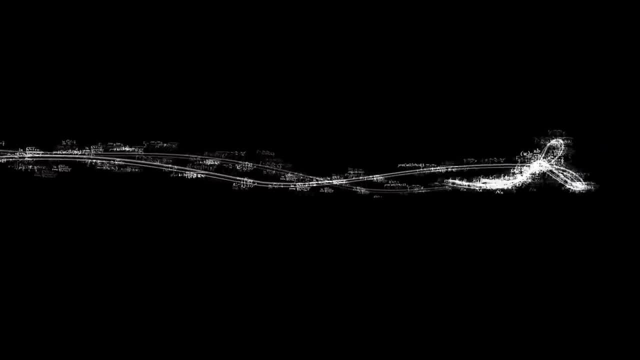 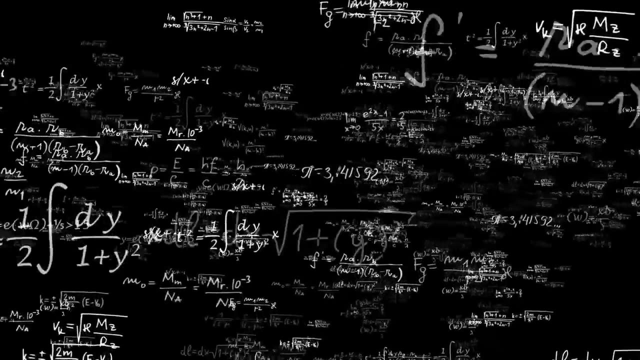 this gave you an idea of the power and intuition behind these things that I think for most people are very dry when we learn them in school. And if you've made it this far and want to expand your knowledge further into a variety of topics, I recommend checking out CuriosityStream, the 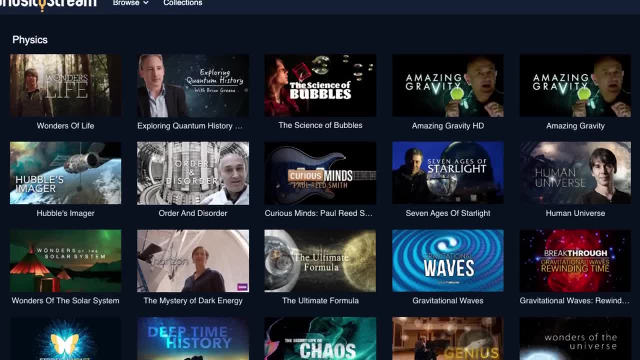 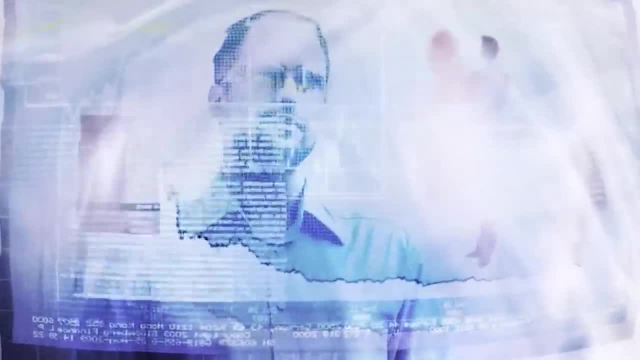 sponsor of today's video. CuriosityStream hosts thousands of documentaries and non-fiction titles put on by industry leaders that you will very likely enjoy if you're a fan of this channel. Watch documentaries like The Hawking Paradox if you want to learn more about one of the greatest.